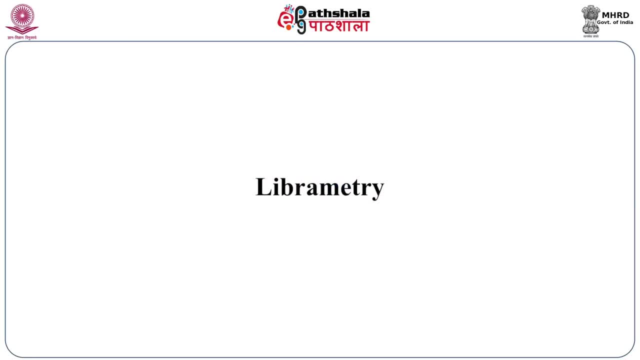 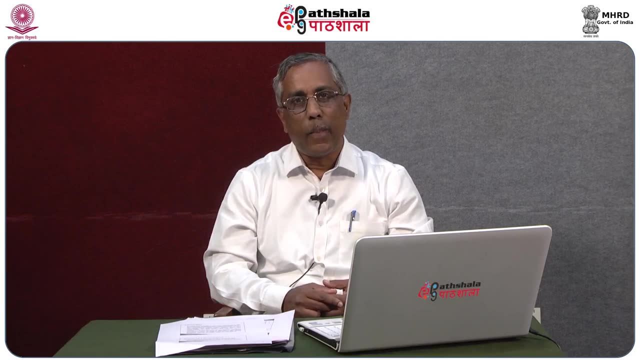 scope and application of Libromatrix. So, Libromatrix, it is a great contribution of Dr S R Ranganathan, Father of Library Movement in India, and we are very proud to inform you that the Bibliomatrix is the the. 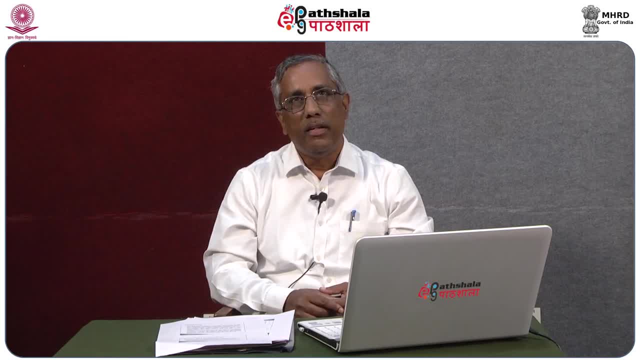 most important tool for research and development in the world. It is a very important tool. So let us begin with the Libromatrix. Let us learn about the term, its meaning and origin is the first of its kind in the world, and after that only the quantitative analysis. 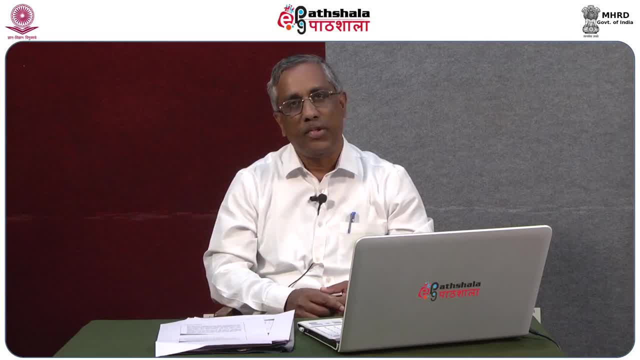 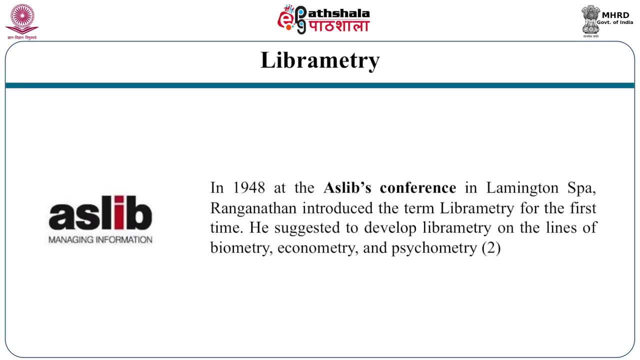 which is applicable to the library and information science have been emerged: LIBRARIMETRY MEANING AND DEFINITION. In 1948, at the ASLIP's conference in Lamington, Spa, Ranganathan introduced the term LIBRARIMETRY for the first time. He suggested to develop 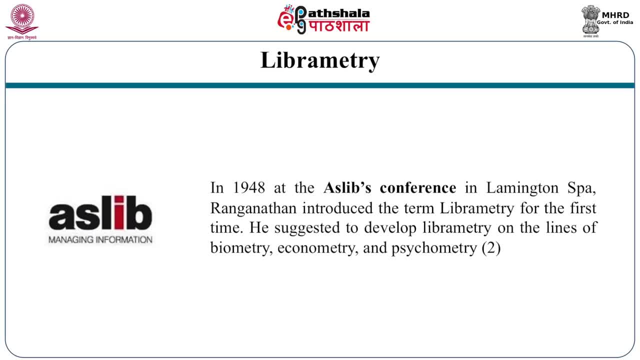 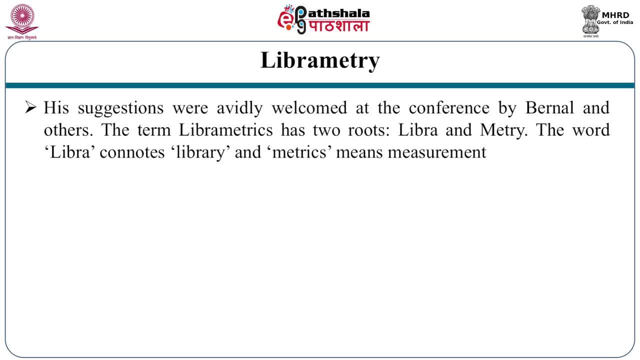 LIBRARIMETRY on the lines of BIOMETRY, ECOMETRY and PHYSIOMETRY. His suggestions were avidly welcomed at the conference by Bernal and others. The term LIBRARIMETRY has two roots: LIBRA and METRY. The word LIBRA connotes LIBRARY and METRIX. 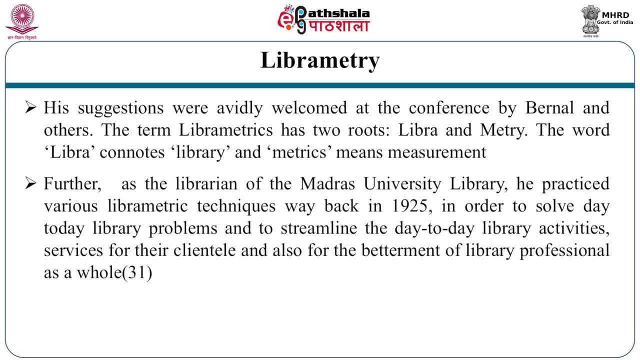 means measurement. Further, as the librarian of the Madras University Library, he practiced various LIBRARIMETRY techniques way back in 1925.. In order to understand LIBRARIMETRY and METRIX in detail, Ranganathan suggested to develop: 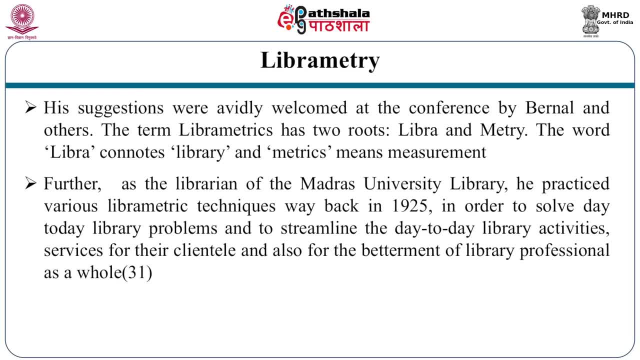 LIBRARIMETRY for the first time in the world. He suggested to develop LIBRARIMETRY for the first time in the world. He suggested to develop LIBRARIMETRY for the first time in the world In order to solve day-to-day LIBRARY problems and to streamline the day-to-day LIBRARY activities. 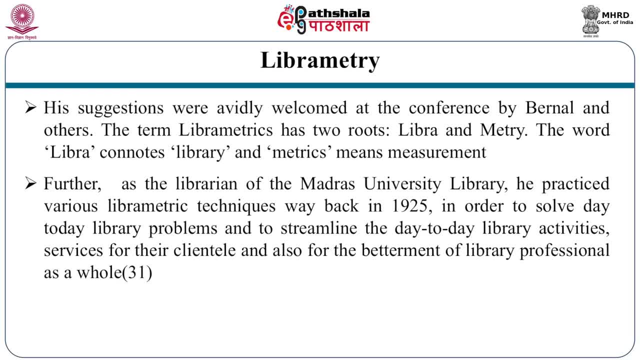 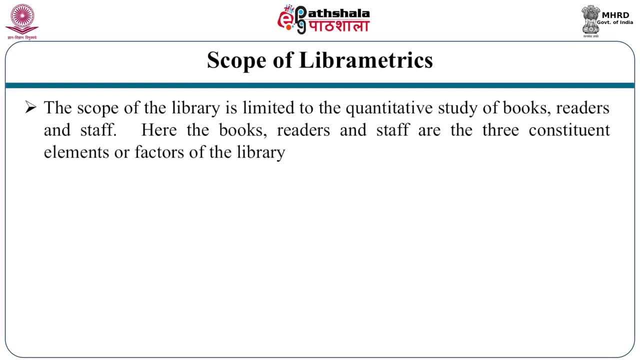 services for their clientele and also for the betterment of the LIBRARY professional as a whole. The scope of the LIBRARIMETRY is limited to the quantitative studies of books, readers and staff. Here the books, readers and staff are the three- constitute elements or factors of. 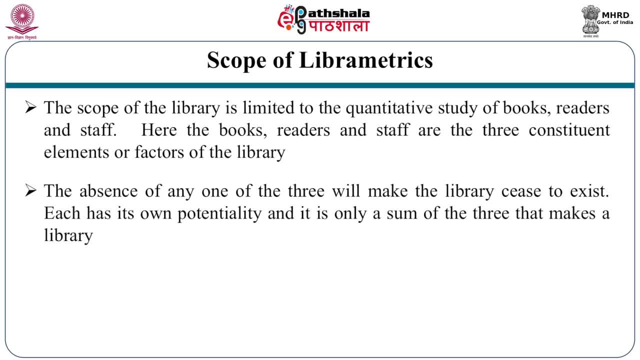 the LIBRARY. The absence of any one of three will make the LIBRARY cease to exist. Each has its own potentiality and it is only a sum of three that makes a LIBRARY. Thus we can measure all the characteristics of books, readers and staff. 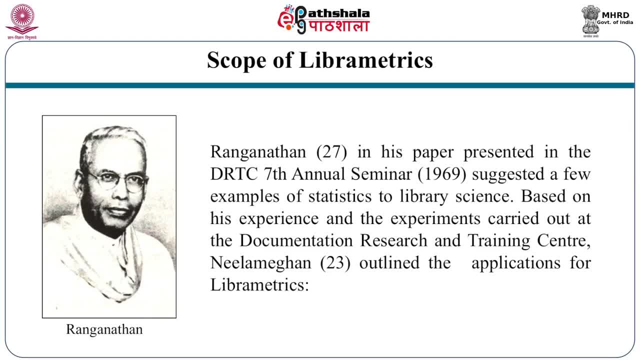 APPLICATION FOR LIBRARIMETRIX. Ranganathan, in his paper presented in the DRTC's 7th Annual Seminar, 1969, suggested a few examples of statistics to LIBRARIMETRY Based on his experience and the experiments carried out at the Documentation, Research and Training Center. 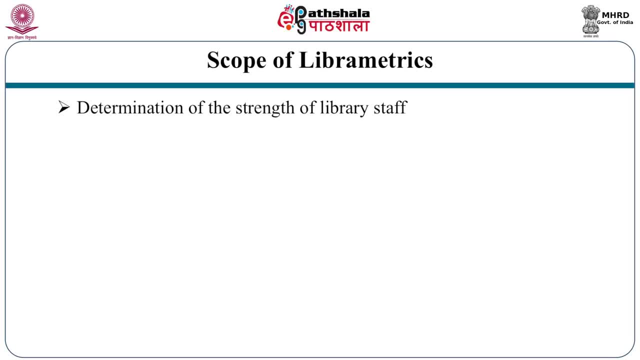 outline the application for LIBRARIMETRIX: 1. Determination of the strength of LIBRARY staff. 2. Disposition of LIBRARY staff for circulation work during different LIBRARY hours. 3. Disposition of LIBRARY staff for reference service during different LIBRARY hours. 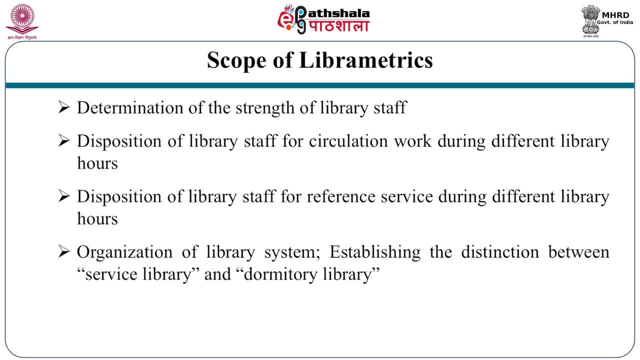 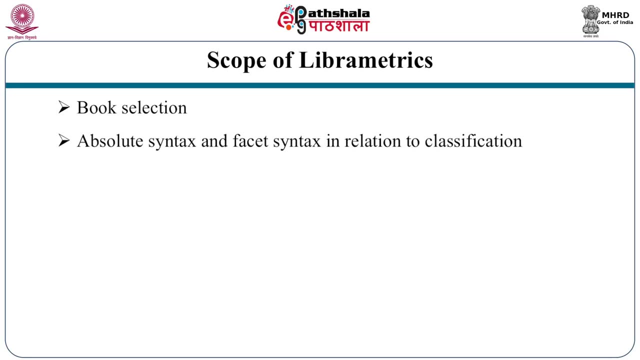 4. Organization of LIBRARY systems. 5. Design of LIBRARY buildings, fittings and furniture. 6. Book selection. 7. Absolute syntax and facet syntax in relation to classification. 8. Length of class number. 9. Variation in style. in writing. catalog entries. 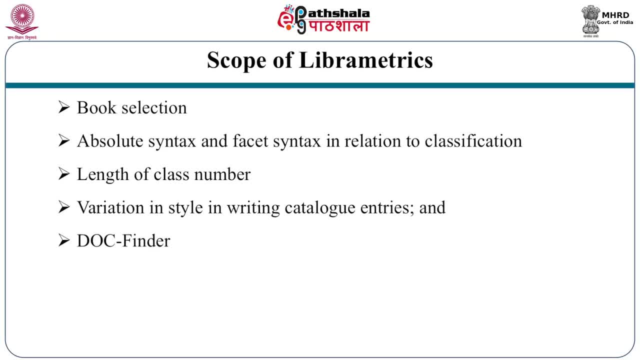 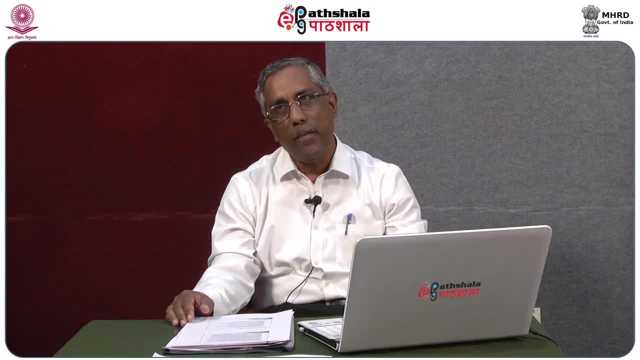 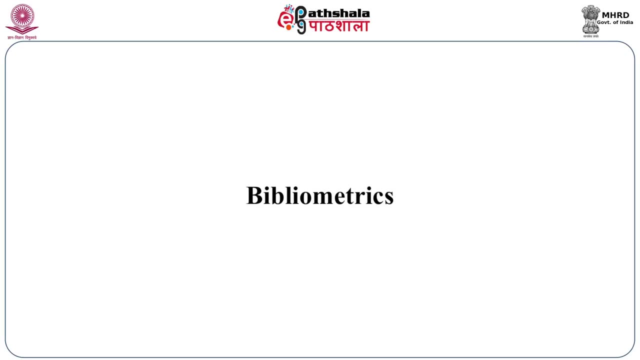 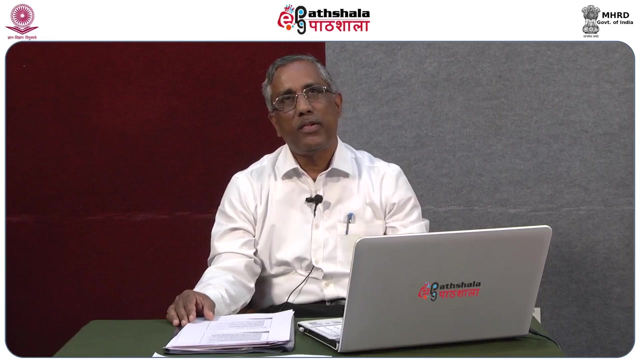 10. DOC Finder. So far we have seen about LIBRARIMETRIX. It is time to see the BIBLIOMETRIX. The BIBLIOMETRIX differs from LIBRARIMETRIX. LIBRARIMETRIX is restricted to a particular library. 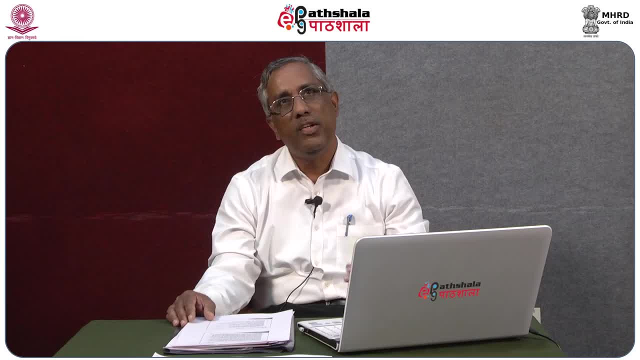 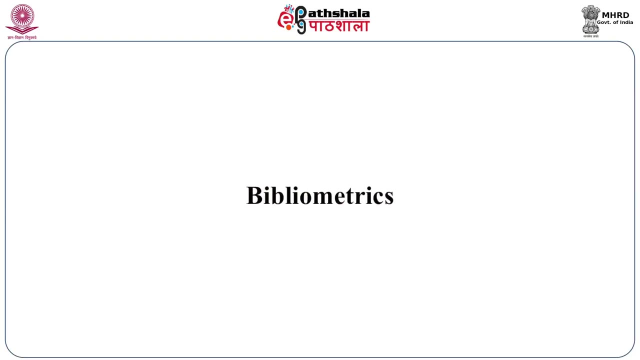 Whereas the BIBLIOMETRIX is in general, LIBRARIMETRIX is restricted to a particular library. Whereas the BIBLIOMETRIX is, in general, about the quantitative aspect of communicated written materials in the books and journals. Bibliometrics- 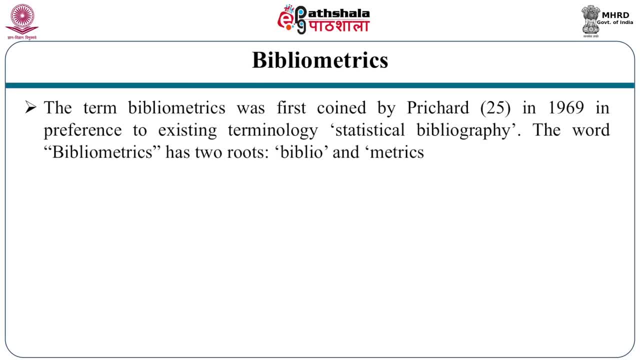 The term bibliometrics was first coined by Pritchard in 1969, in preference to existing terminology Statistical Bibliography. The word bibliometrics has two roots: biblio and metrics. The term biblio is derived from the combination of Latin and Greek word biblion, equivalent to bylos, meaning book, paper, which in turn was derived from the word bylos, a city of Phoenicia, a noted city for export trade in paper. 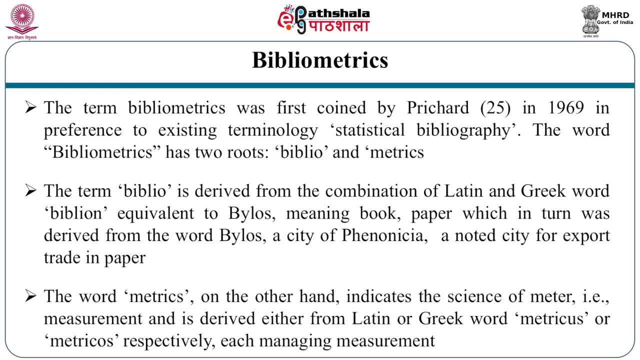 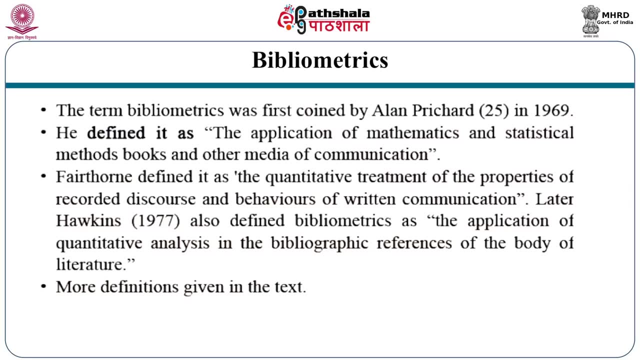 The word metrics, on the other hand, indicates the science of meter, that is, measurement, and is derived either from Latin or Greek word metricus or metricos respectively, is managing measurement. This term was coined for the first time by Alan Pritchard. 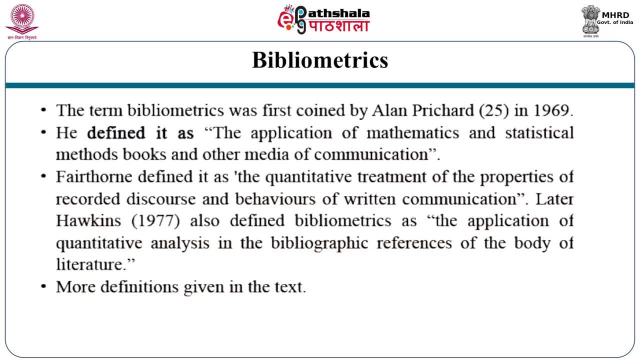 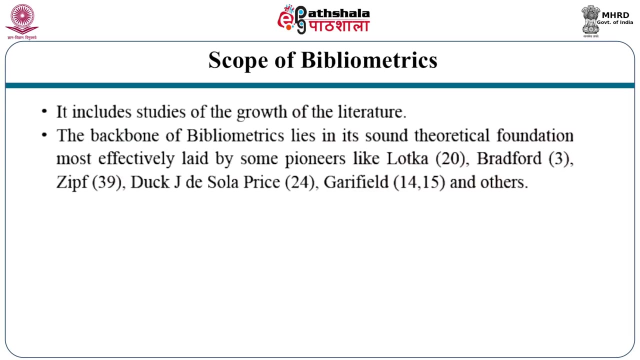 He used the term to describe all studies which seek to quantify the process of written communication. Phaethon also defined it as the quantitative treatment of the properties of recorded discourse and behavior pertaining to it. Scope of Bibliometrics: Bibliometric studies include studies of the growth of the literature in some subject. 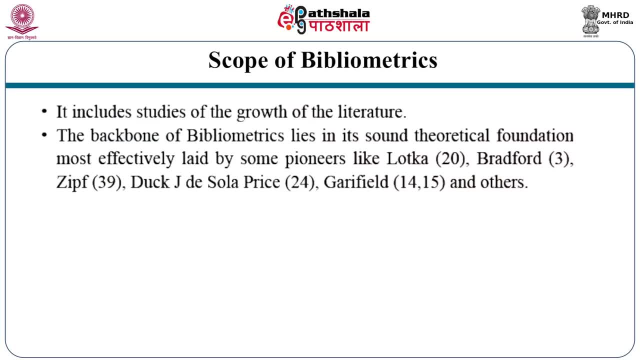 how much literature is contributed by various individual groups or organizations or countries, how much exists in various languages, how the literature on some subject is scattered and how quickly the literature on some subject becomes out of date. Another important point is that another important group of bibliometric studies relate to word source, author side. 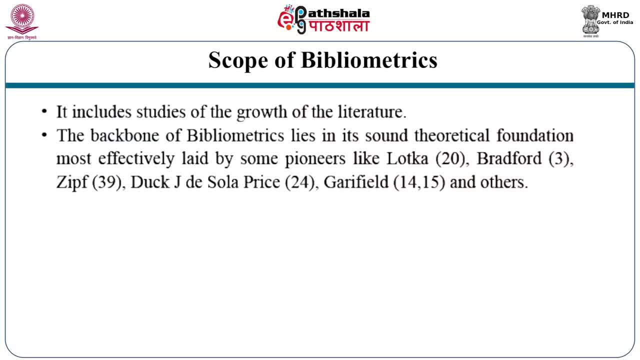 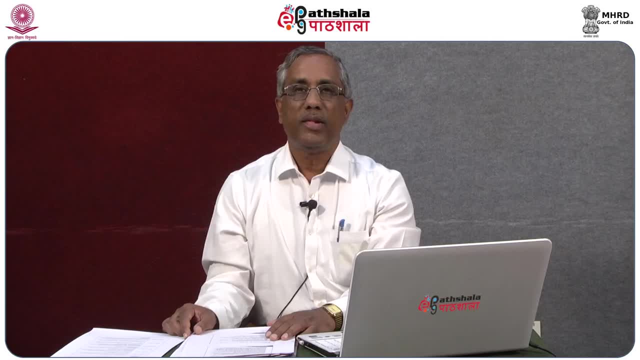 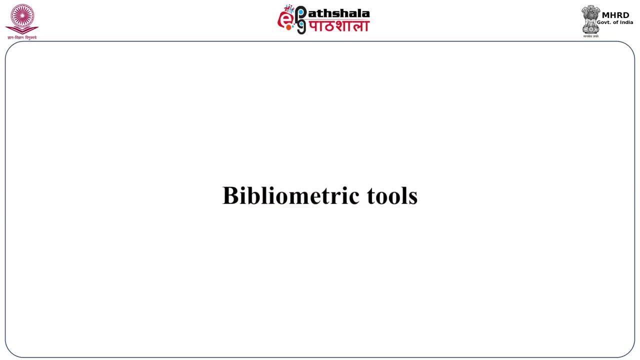 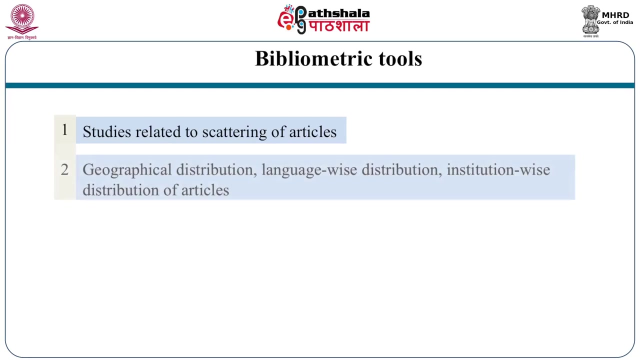 Day by day. this study is attaining sophistication and complexity, having national, international and interdisciplinary character. Now we can see the bibliometric tools. how can be applied to the library and information science activities? Studies related to scattering of articles. Secondly, geographical distribution: language wise distribution. 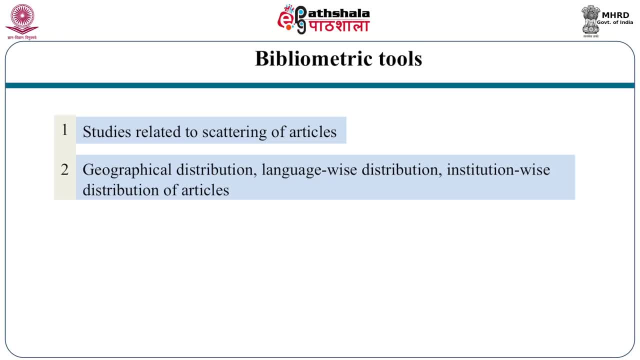 institution: wise distribution of articles. Third, age distribution of documents. Fourth, distribution of citations: subject, author, language, type, journal, etc. Fifth, use of information storage and retrieval. Sixth, application in the library use studies. Seventh, to study the trends in research and identifying the growth of literature. 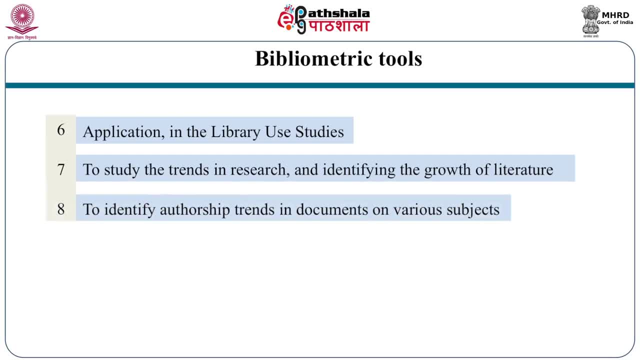 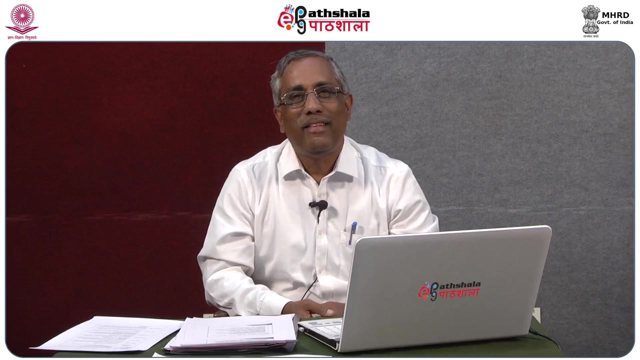 Eighth, to identify authorship trends in documents on various subjects. Ninth, to measure the utility of library services. Tenth, to evaluate library collection, etc. When we compare the librometrics and the bibliometrics, librometrics is restricted to a particular library. 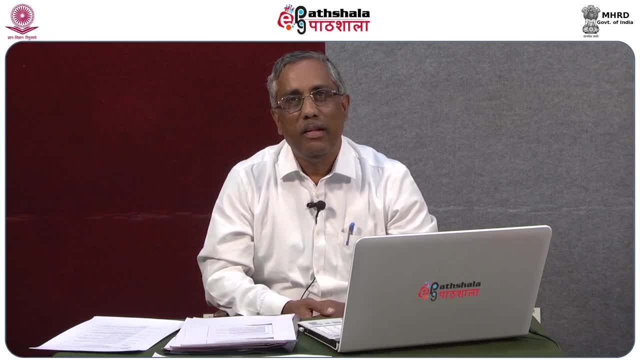 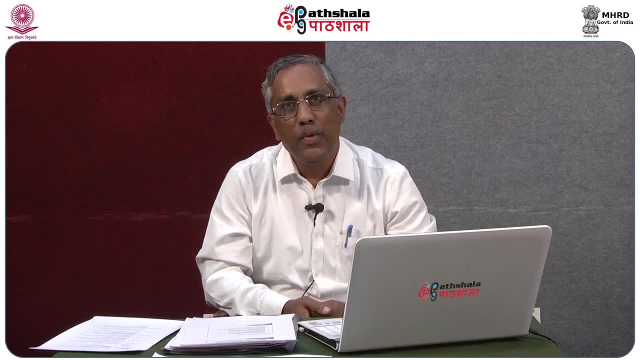 whereas bibliometrics is in general, studies the quantitative aspects of communicated literature in the field of library and information science. And here we can see the various aspects of communicated literature may be its form, may be its type, may be its language. 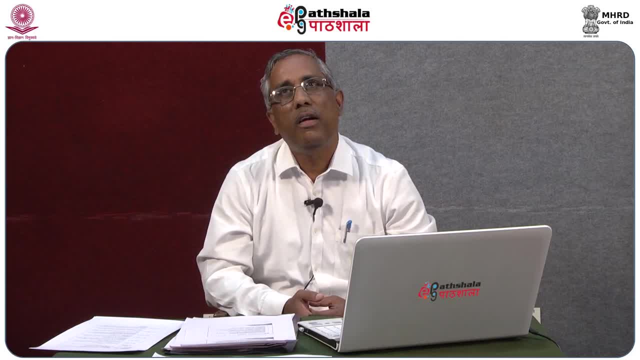 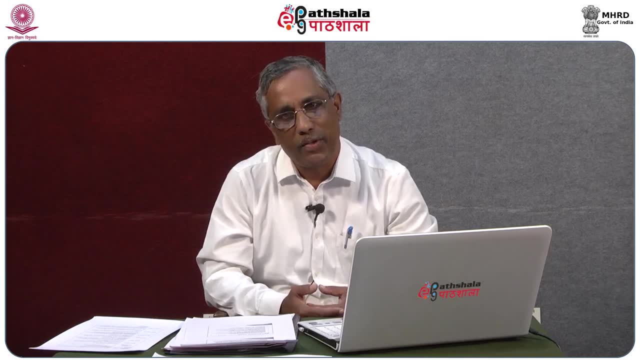 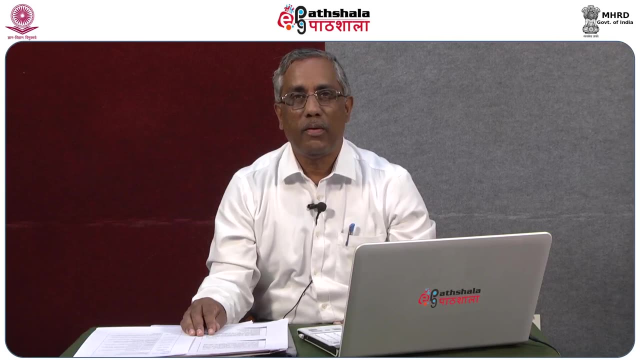 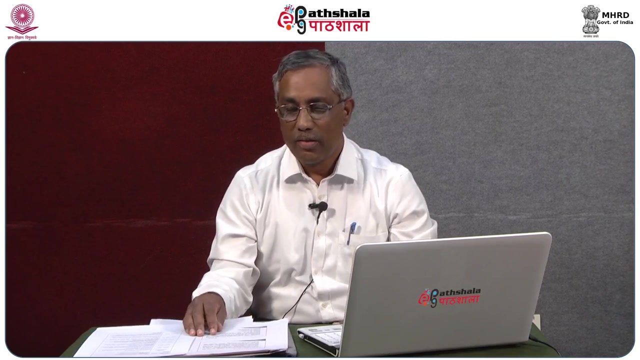 may be a particular country, or even how actually it has been communicated in the different subjects. That also we can study here. Friends, so far we have discussed librometrics and bibliometrics. Now let us discuss about scientometrics. Scientometrics, the term. 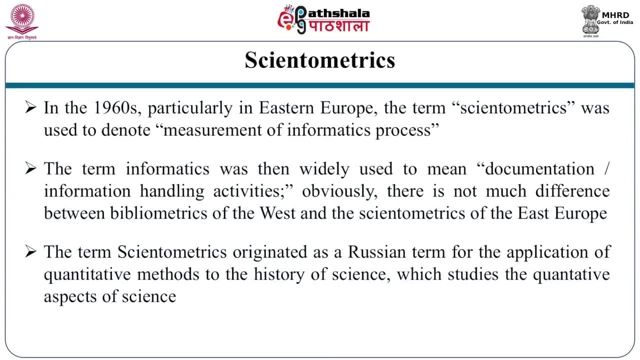 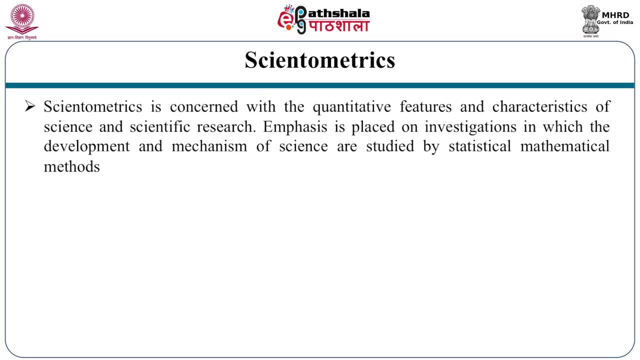 originated as a Russian term for the application of quantitative methods to the history of science, which studies the quantitative aspect of science. Scientometrics is considered with the quantitative features and characteristics of science and scientific research. Emphasis is placed on investigation in which the development and mechanism of science 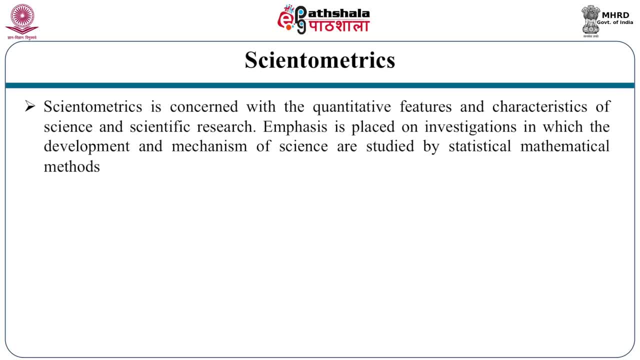 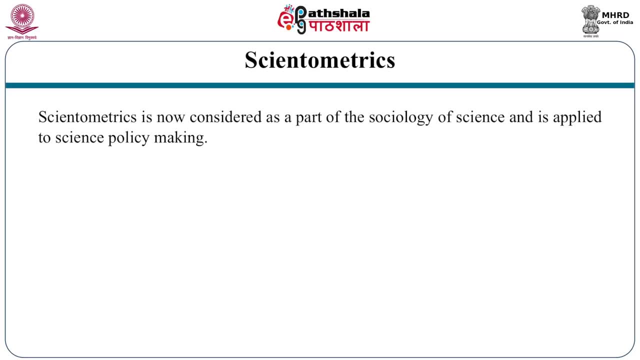 are studied by statistical mathematical methods. Scientometrics is now considered as part of the sociology of science and science applied to science policy making. Thus, scientometrics involves studies in sociology of science, history of science, growth of literature, behavior of scientists. 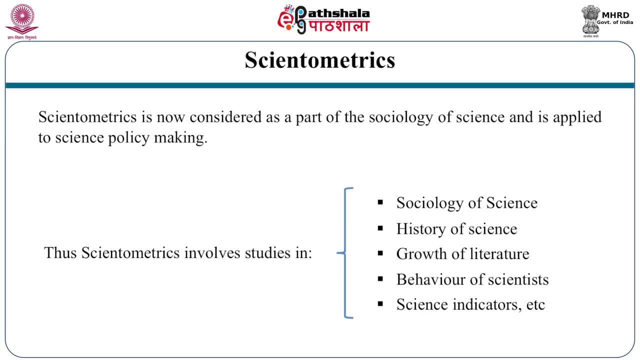 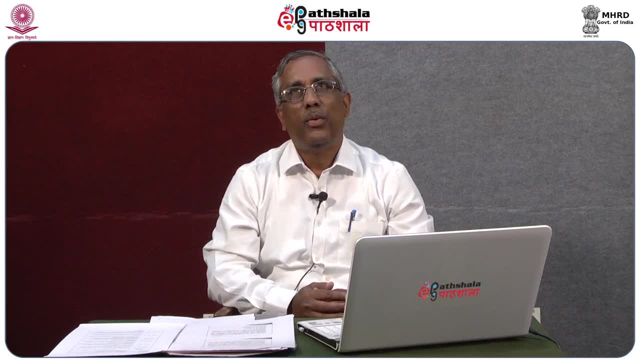 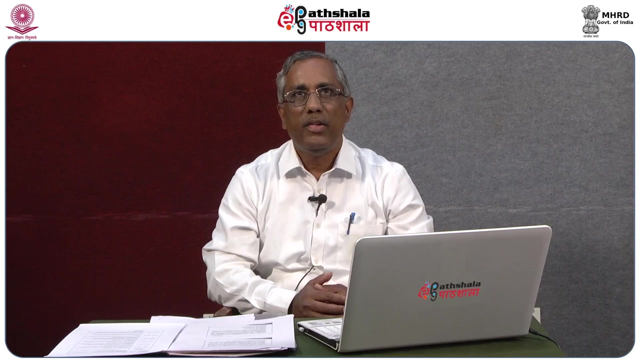 science indicators, etc. Friends, I can put it in brief. Scientometrics is actually a tool which has been used by Westerners specifically to study history of science And most of the European countries- nowadays they are having history of science institutes. 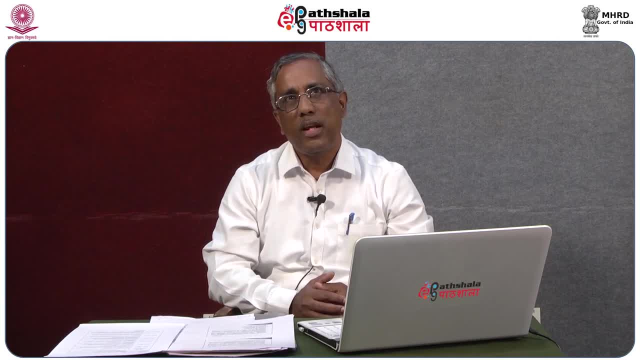 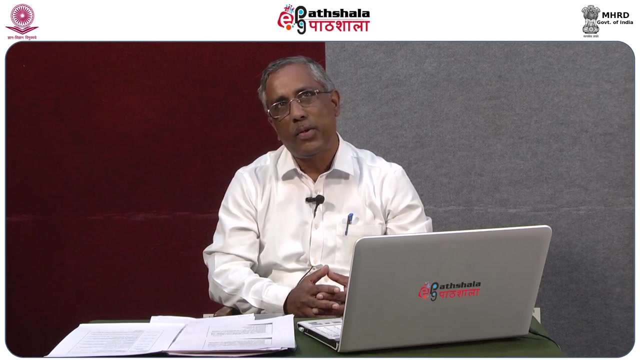 With help of that history of science institutes, they are able to give many indicators for their science and technology subjects And specifically, De Sola-Frice has given much importance to the scientometrics. And when you think about scientometrics, but even though it looks like similar to the 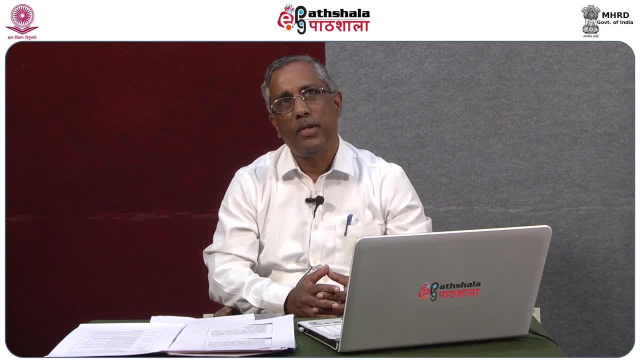 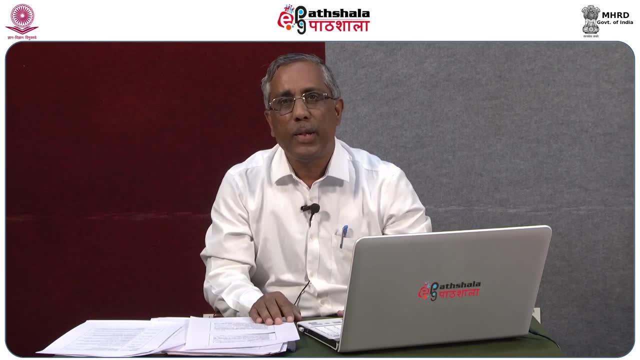 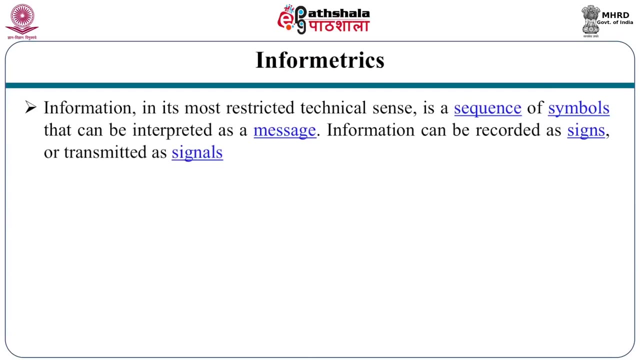 similar to the librometrics and bibliometrics, but it is similar but not same. So far, you have studied librometrics, bibliometrics and scientometrics. Now let us move to informetrics. Information in its most restricted technical sense. 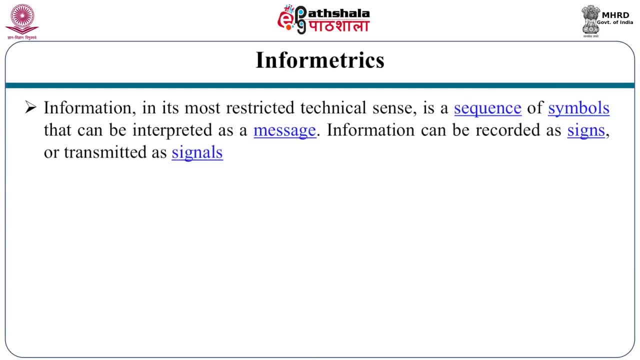 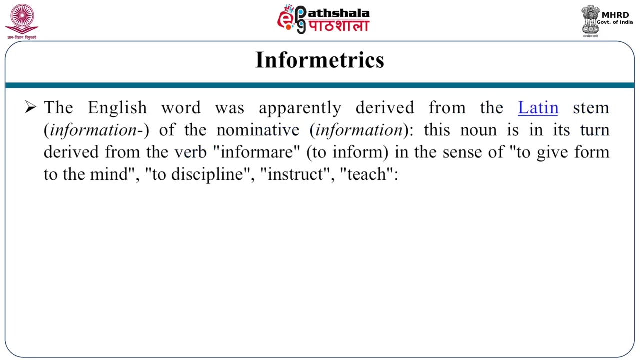 is a sequence of symbols that can be interpreted as a message. Information can be recorded as signs or transmitted as signals. Information is any kind of event that affects the state of dynamic system. Conceptually, information is the message being conveyed. The English word was apparently derived from: 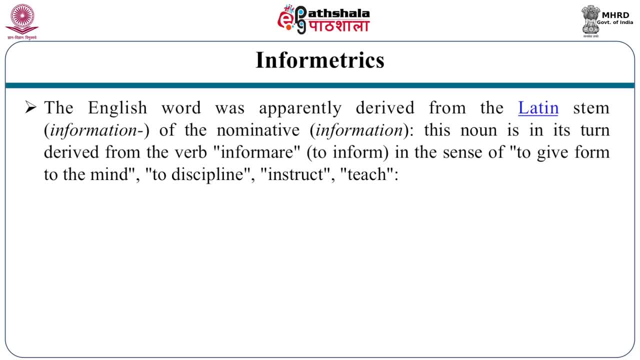 the Latin stem, information, of the nominative information. This noun is in its turn derived from the verb informere, to inform In the sense of to give form to the mind, to discipline, instruct or teach. Metrics means measuring. Informetrics is the study of quantitative aspect of information. 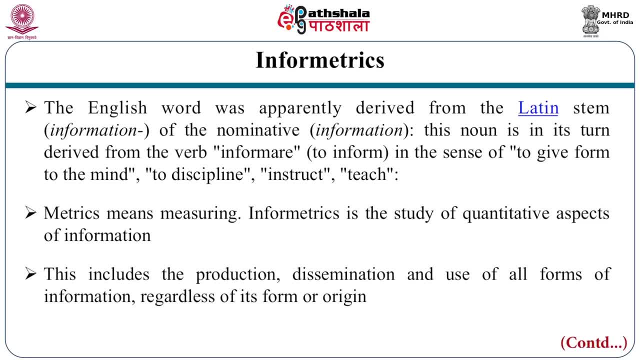 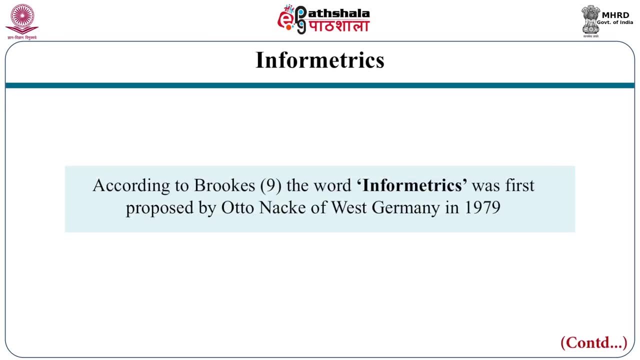 This includes the production, dissemination and use of all forms of information, regardless of its form or origin. According to Brooks, the word informetrics was first proposed by Otto Necke of West Germany in 1979.. Then FID constituted a committee. 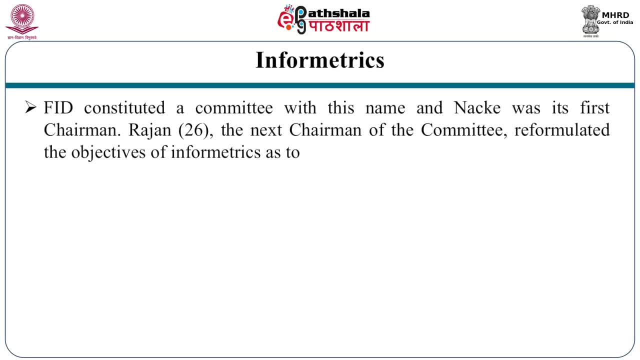 with this name, and Necke was its first chairman. then Rajan, the next chairman of the committee, Re-formulated the objectives of informetrics as provide reliable data for research and development, policy making and planning, To evaluate institutions, projects, articles, products. 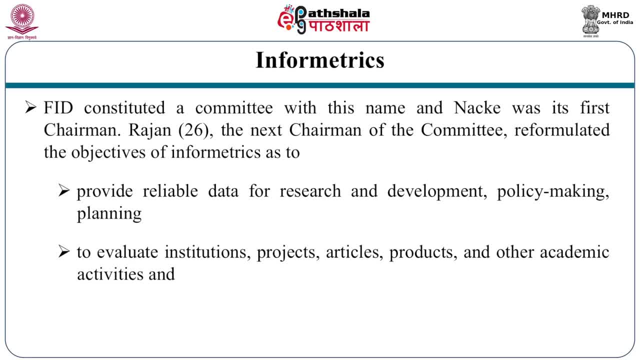 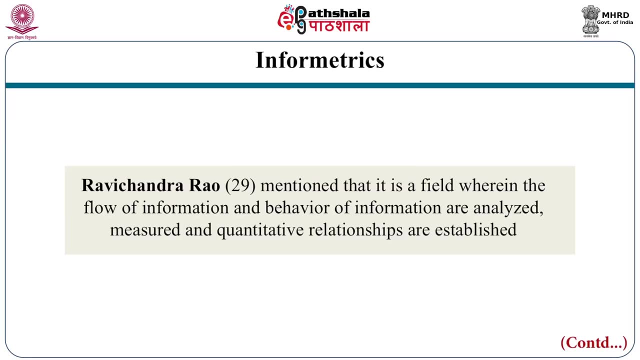 and other academic activities, And to identify or to develop the techniques or trace the origins and development of concepts. Dr Rajchandra Rao mentioned that it is a field wherein flow of information and behavior of information are analyzed, measured and quantitative relationships are established. 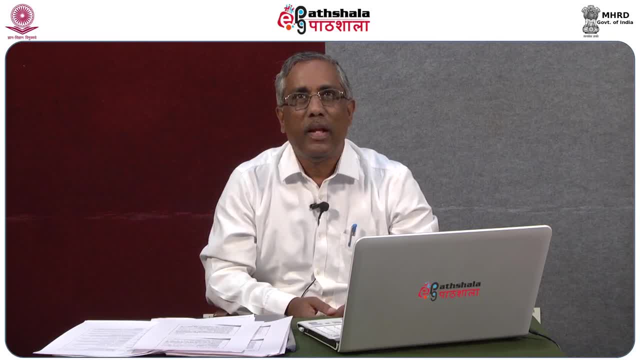 In brief, I can summarize like this: Liberometrics, related to library, bibliometrics, related to communicative aspects of communicated literature, and scientometrics is a term derived from the Russian language and which is science of science. Informetrics is derived from the word information. 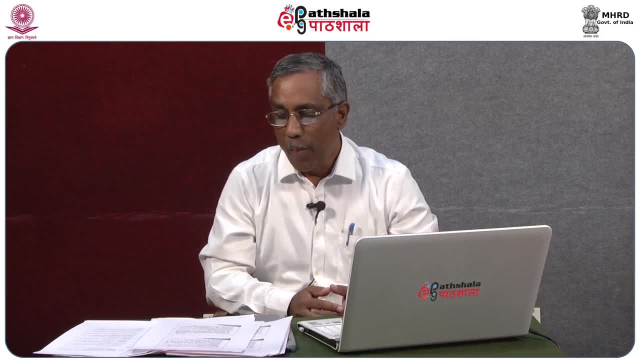 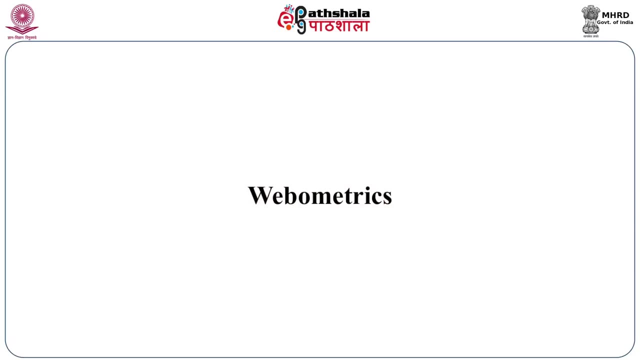 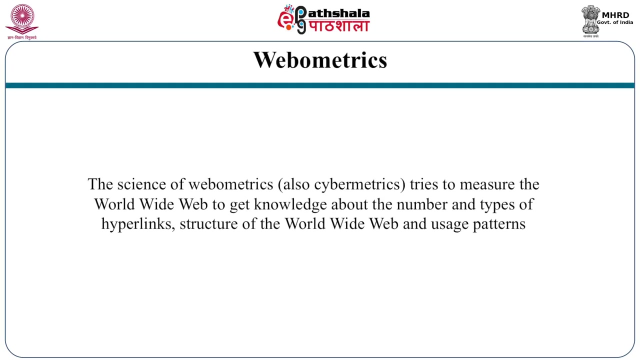 which is very much useful from the point of view of analyzation of the information and measuring of the quantity of information. Friends, now let us turn to the web-o-metrics and cyber-metrics. Both are similar but having little different. The science of web-o-metrics. 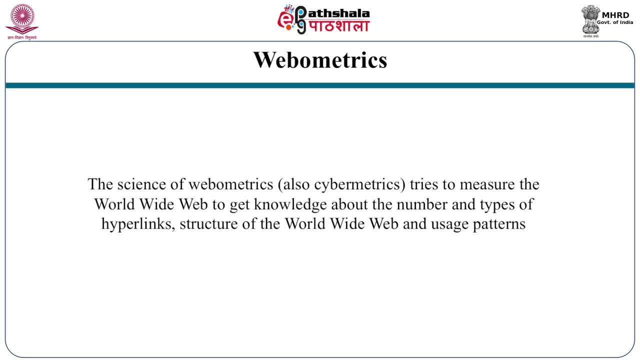 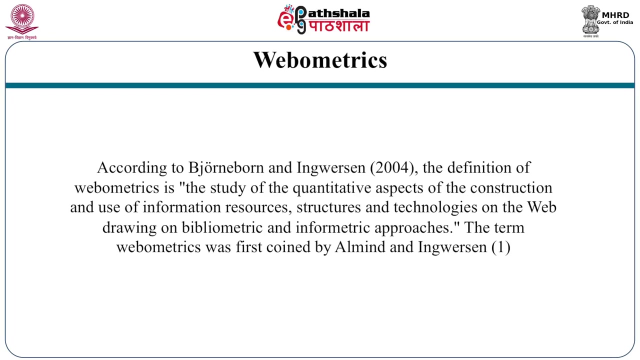 also we can call cyber-metrics. Cyber-metrics tries to measure the world wide web, to get knowledge about the number and types of hyperlinks, structure of the world wide web and usage patterns. According to Bjorn Bern and Ivingson, the definition of web-o-metrics 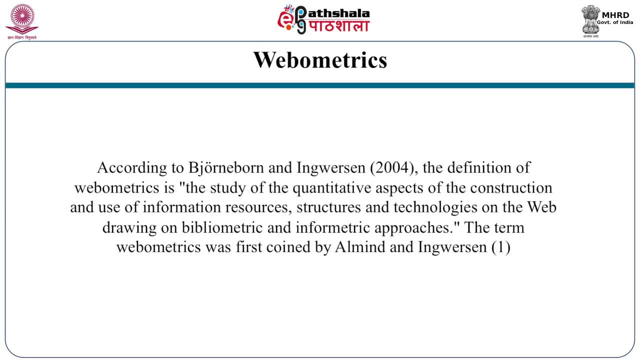 is the study of the quantitative aspect of the construction and usage of information resources, structures and technologies in the web, drawing on bibliometrics and informetrics approaches. The term web-o-metrics was first coined by Almond and Ingersoll. The second definition of web-o-metrics. 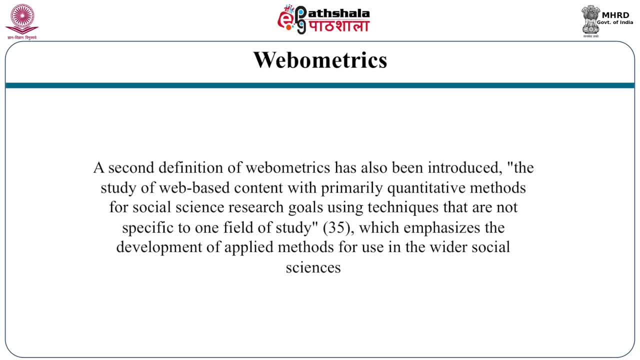 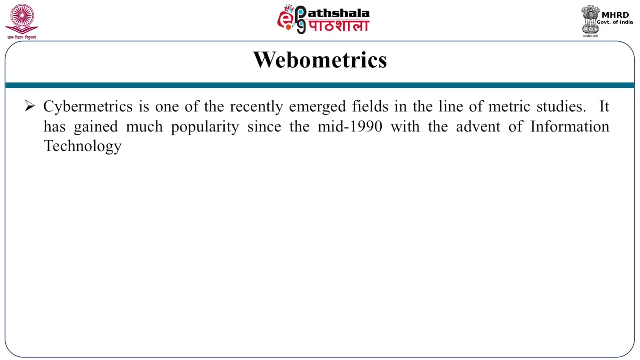 has also been introduced: The study of web-based content with primarily quantitative methods for social science research goals, using techniques that are not specific to one field of study, which emphasizes the development of applied methods for use in the wider social science. Little bit we can see about cyber-metrics. 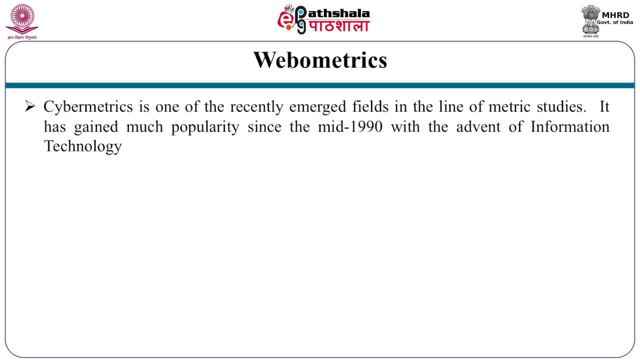 Cyber-metrics is one of the recently emerged fields in the line of matrix studies. It has gained much popularity since the mid 1990 with the advent of information technology. As it is mainly concerned with computer science based approaches, it has superseded all the other matrix studies. 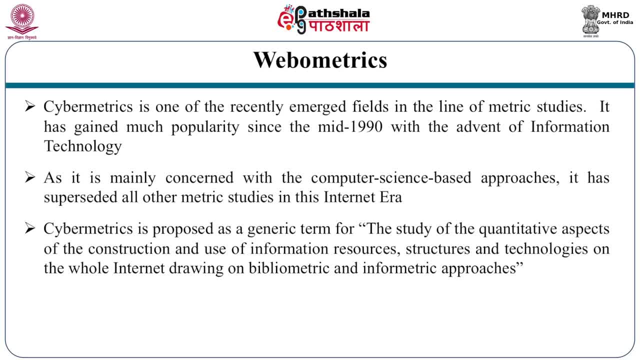 in this internet era. Cyber-metrics is proposed as a generic term for the study of quantitative aspect of the construction and use of information sources, structures and technologies on the whole internet, drawing on bibliometrics and informetrics approaches. Cyber-metrics thus encompasses statistical studies. 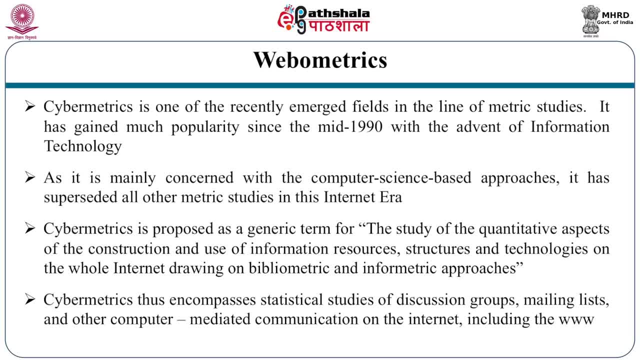 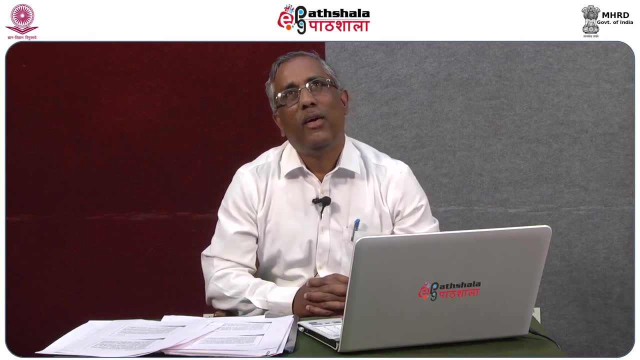 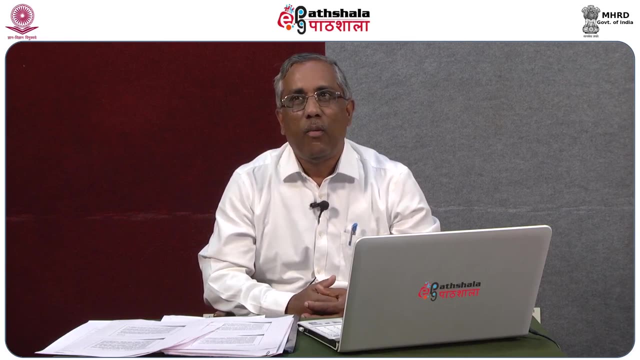 of discussion groups, mailing lists and other computer mediated communication on the internet, including world wide web. I can group or I can make here two parts of the quantitative analysis studies. here What first four we have studied, studied librometrics, bibliometrics, informetrics.